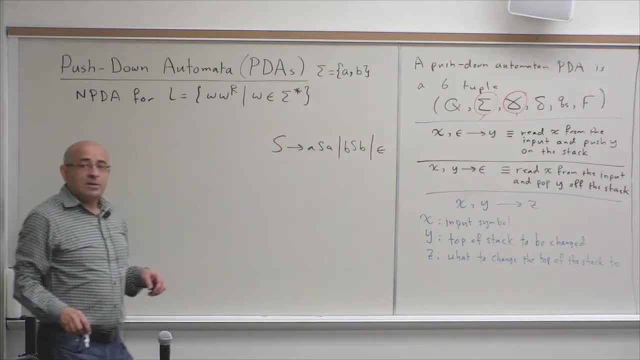 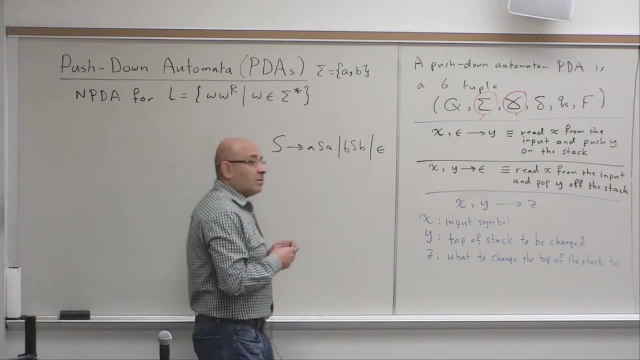 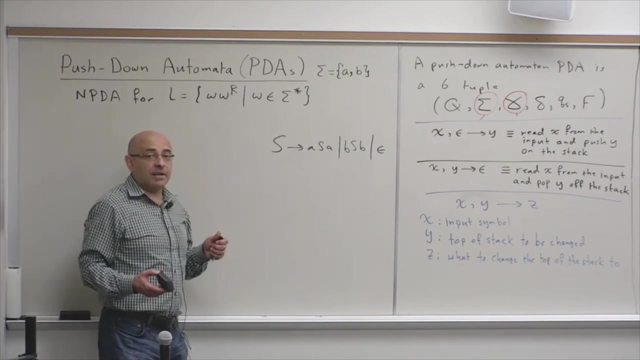 Or epsilon. So this is a grammar. So a grammar generates a language. A PDA recognizes a language, So grammars generate context-free. grammars generate context-free languages. PDAs recognize context-free languages. Now what did we learn for generating regular languages? 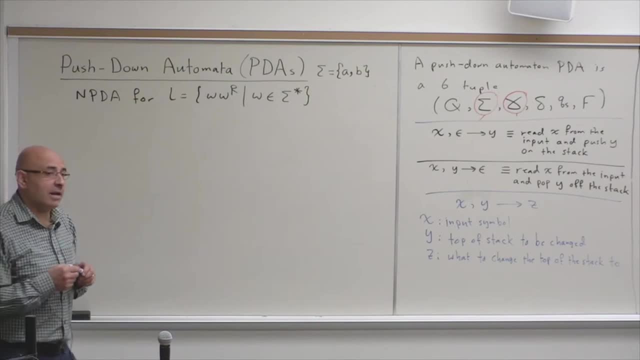 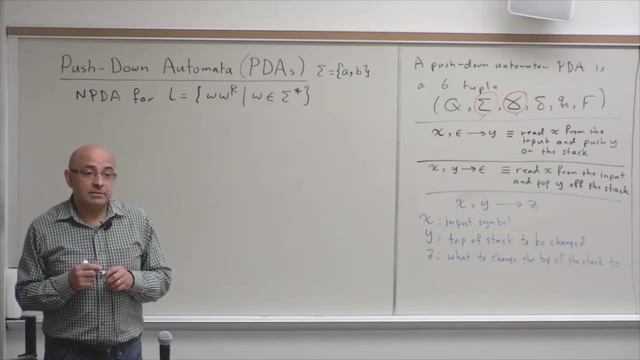 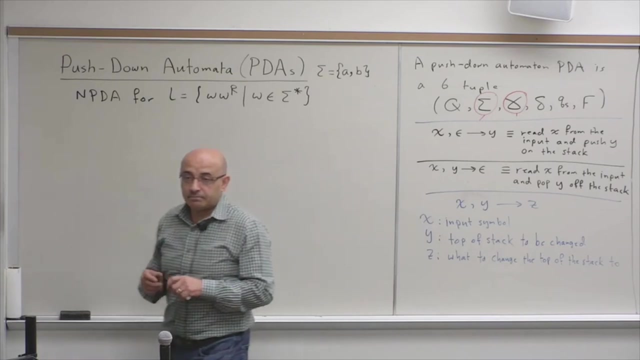 So what are the techniques that we learned for generating regular languages? Yeah, regular expressions and regular grammars as well, So you can generate a regular language using a regular expression or a regular grammar. Okay, So now we need to push down automaton for this. 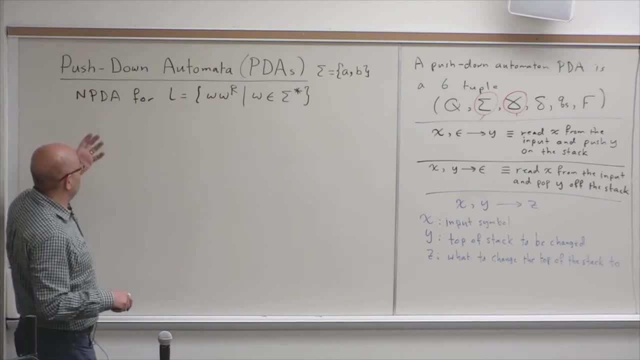 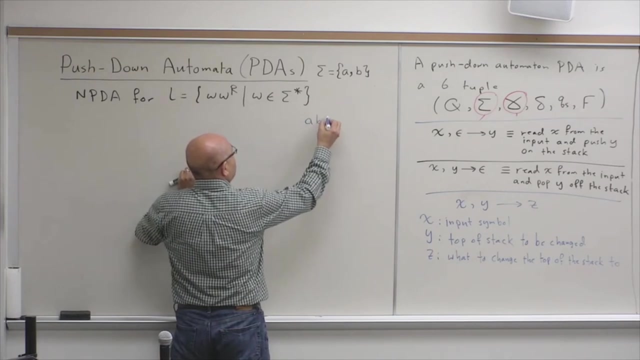 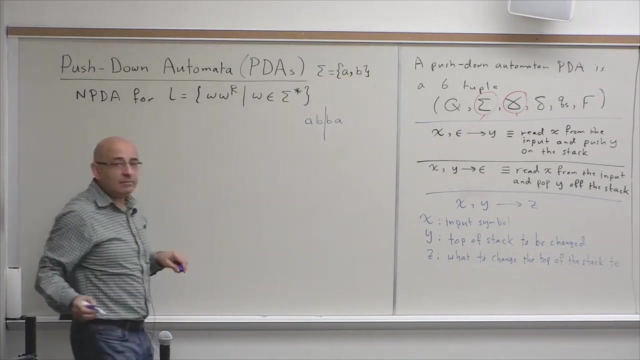 So the idea is very simple. It's very simple. In fact, it's very similar to that, But here, here, we need to match. It's like- let's take an example- string like ABBA. So we need to, we need to use the stack. 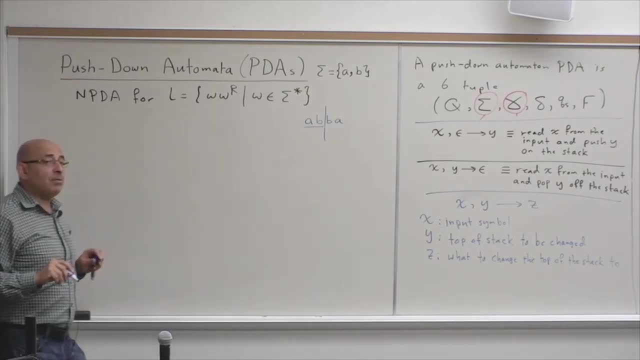 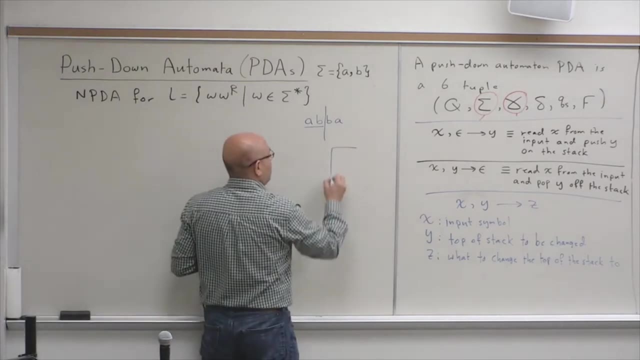 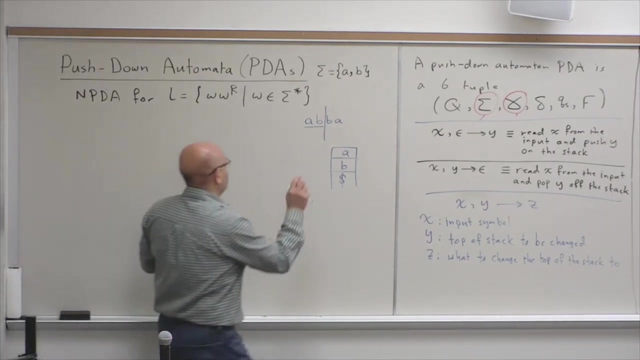 We push this on the stack, Then when we pop, what should we get? So like when we when we push these, so we're going to have A, B pushed on the stack. Sorry, we'll first. okay, so we'll first push the A Then. 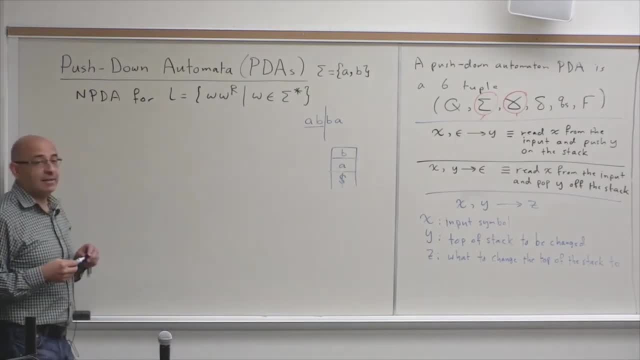 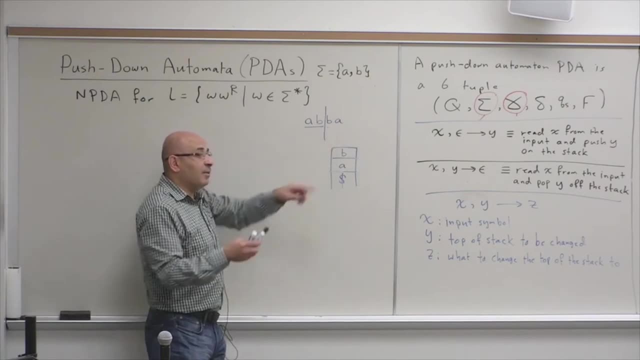 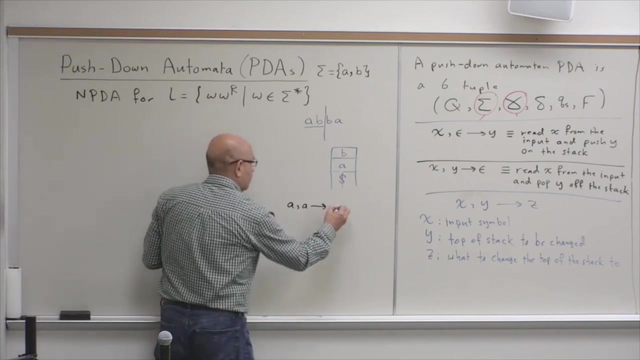 we'll push the B. Then when we pop it should be the same, It should match What we pop, should match what we are seeing at the input. So we will have lots of transitions where you know A, A goes into epsilon and BB goes into epsilon. 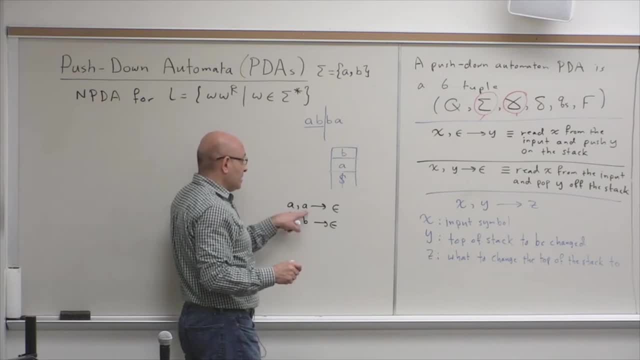 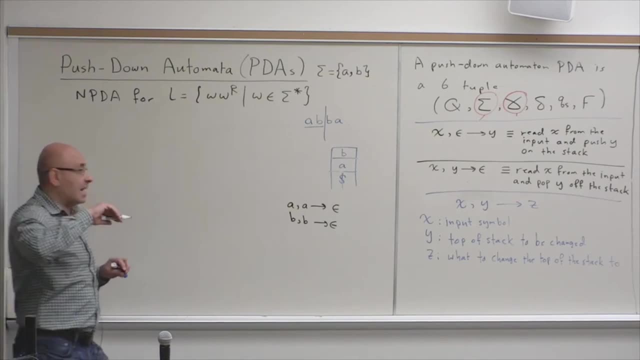 So this is what we are seeing at the input. This is the top of the stack, So the input and the top of the stack should match now, unlike the previous example. So in fact it's going to look the same, but except. 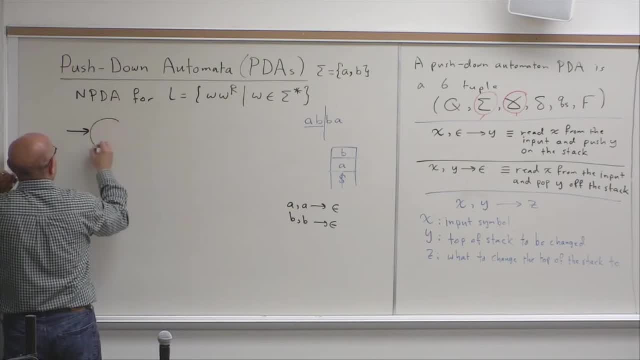 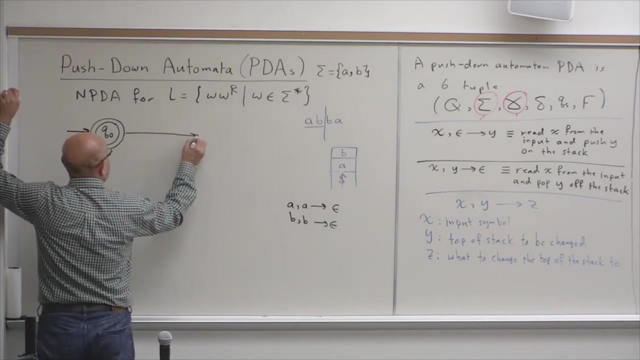 that the transitions are going to be like this. So this is my Start state, which is an accept state, because epsilon belongs to this, and then I have my the same initialization: Nothing, nothing. I'm going to put a dollar sign. 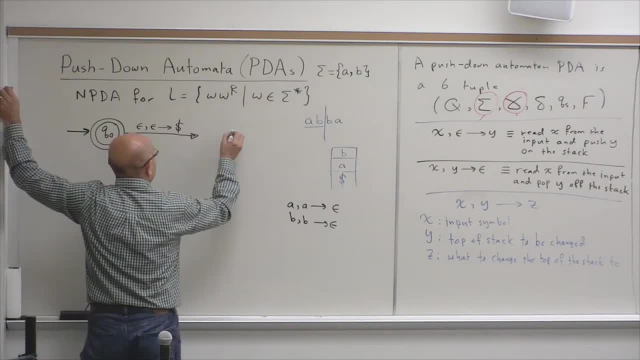 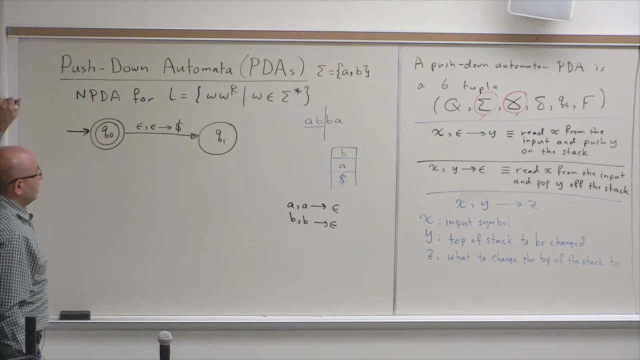 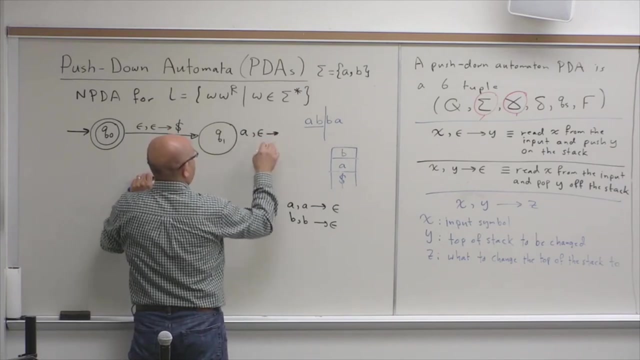 so that I can recognize an empty stack. Now I have a Q1.. Now what should I do? Push or pop, Push, Push anything. So if there is an A, then I push, regardless of what's on the top of the stack. I push an A If there is a B. 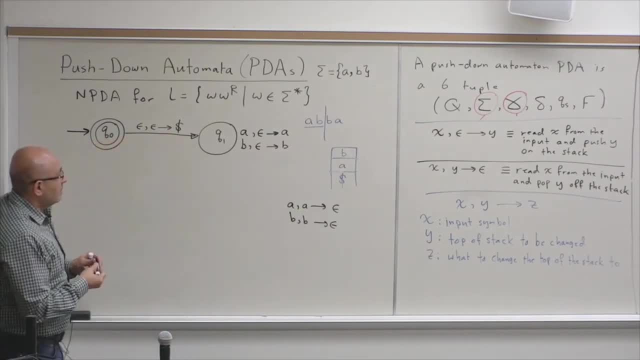 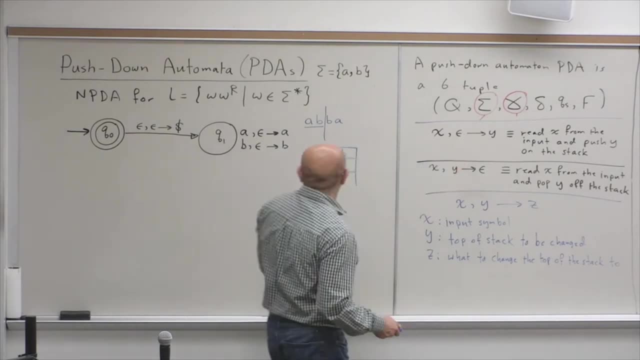 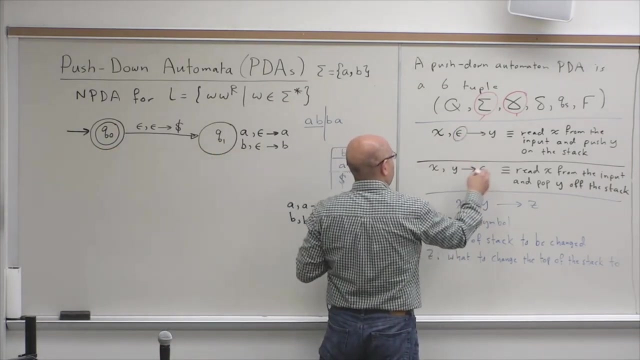 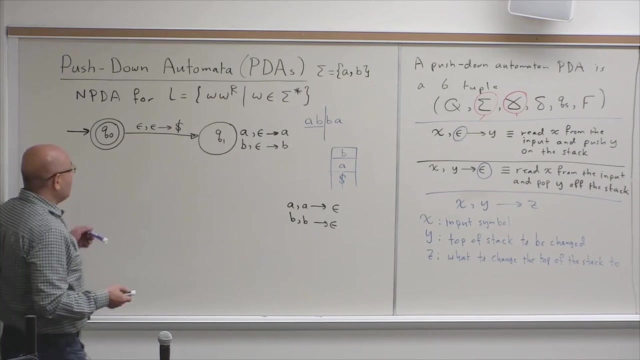 I push a, B. Remember this thing: Read X from the input and push Y. So when you have this epsilon, this is a push. When you have Y goes to epsilon, this is a pop. Now, how do I know now when to get to switch to the popping mode? 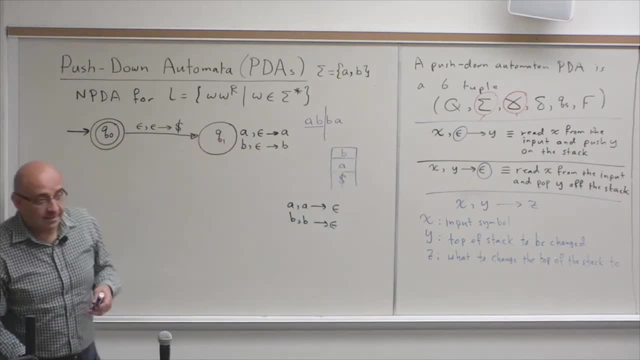 It's a non-deterministic, So I can just put an A. I can do that any time I want. So it's a non-deterministic. It's like an NFA: You make the transition whenever it's the right time for you to. 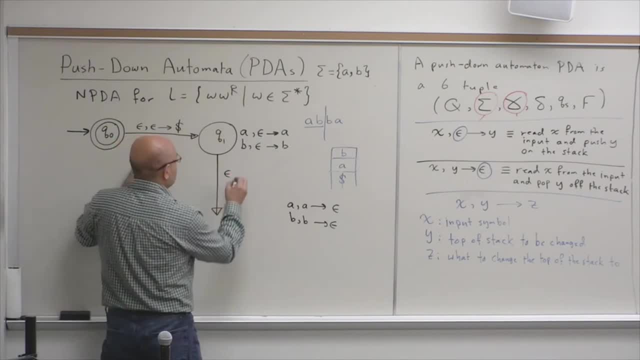 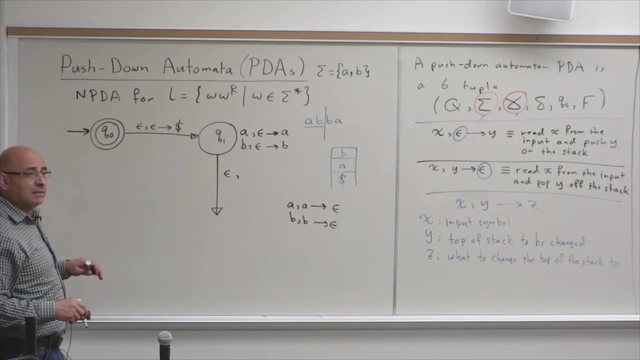 So with an epsilon and what should be the top of the stack? What should be the top of the stack at that point? Nothing, I don't care right. So you can do the. So here you are saying, no matter what I have in the input. 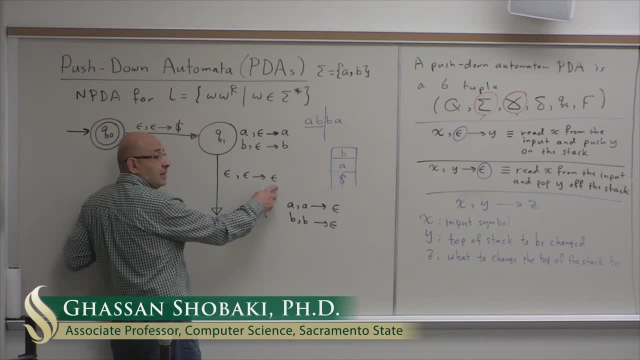 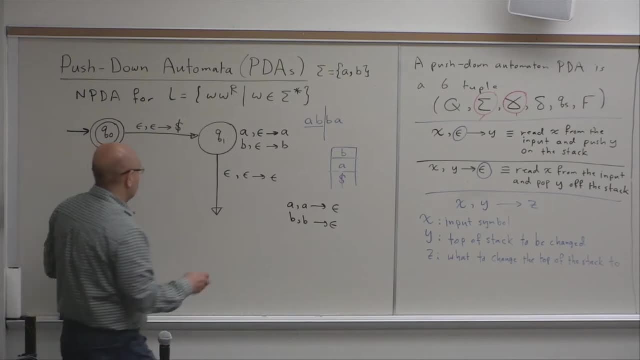 no matter what the top of the stack is, and I'm going to do nothing. It's like a push, nothing. So this is just like a pure epsilon transition And, like I said, you know, in the spring, In non-deterministic finite automata, we take the epsilon transition when it's good for us. 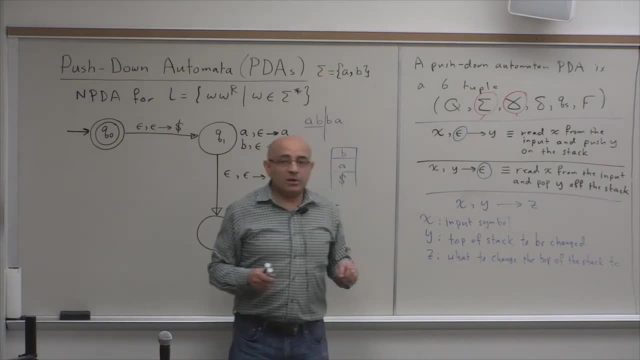 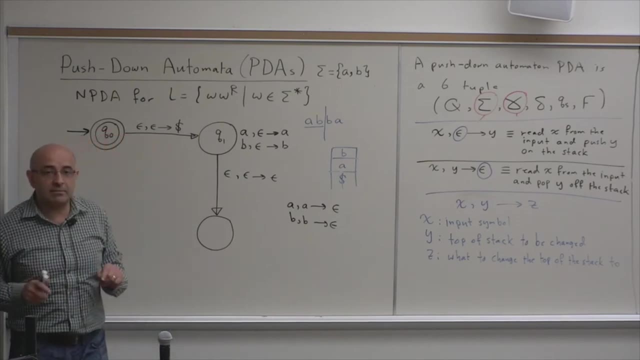 to take the epsilon transition. It's like you know, you are trying to get that string to get accepted, so you choose to take the epsilon transition when it's a good time to take the epsilon transition so that this string gets accepted. Now here what should happen. 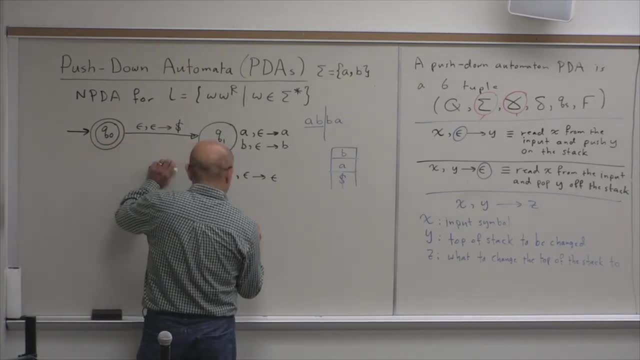 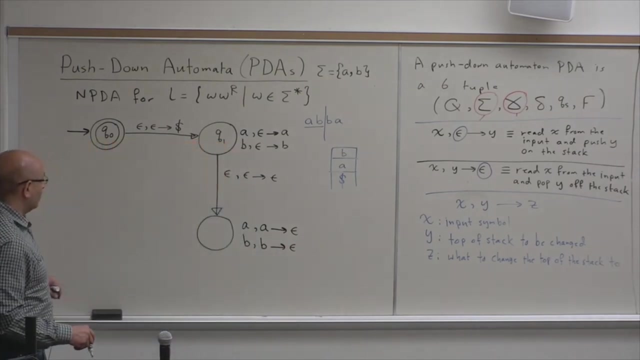 I should pop. Now if I have a, if I'm reading an A, I should pop an A, And when I'm reading a B, I should pop a B, And this is the state Q2.. Now I accept what's the transition. 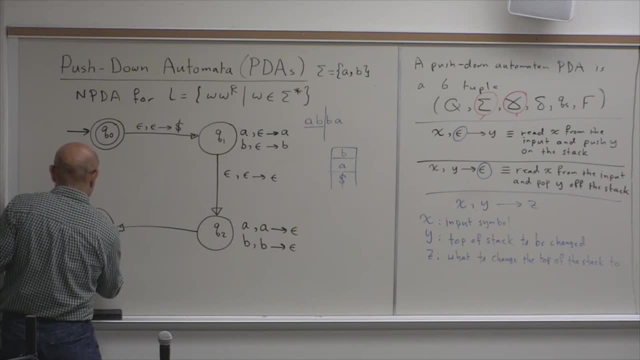 that will put me in an accept state. A, Yeah, so the exactly the at the input. I should have nothing At the top of the stack. I should have a dollar sign and I would. I will pop it And this would recognize the language WWR using this. so again, 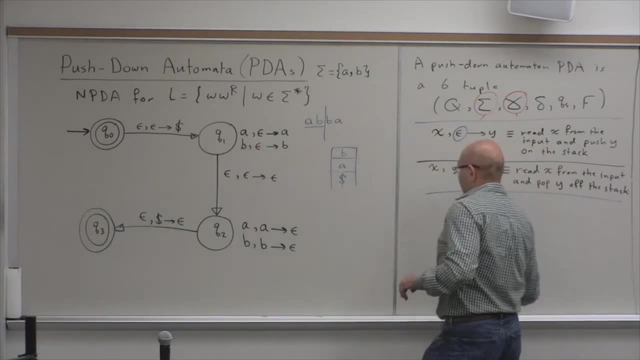 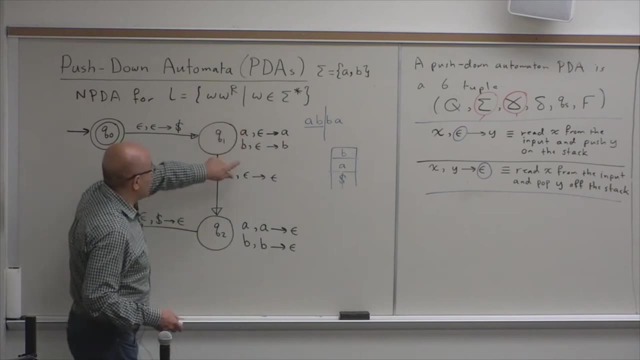 you know clearly, if you have a valid, if you have a valid string like ABBA, you would push these two. You push the A, then you push the B, Then here, when you pop the first time, you pop what You pop: a, B, You pop the same as what you have. 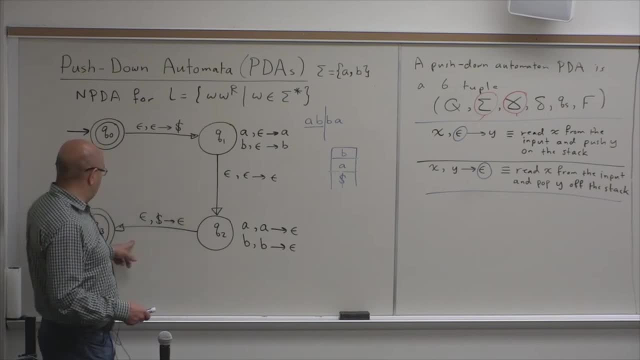 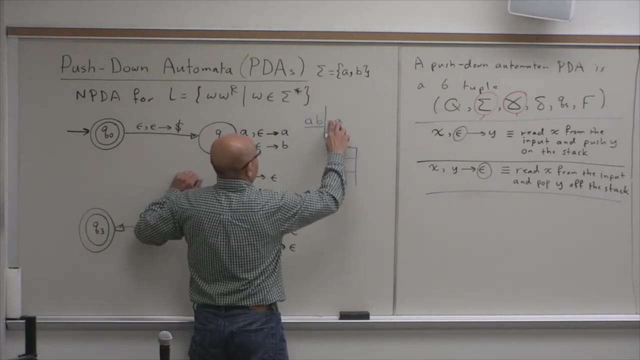 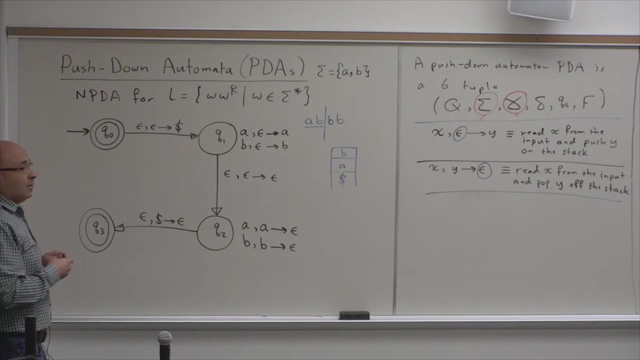 So like if and then you are done and you go to an accept state. Now, if we put a string that doesn't belong to the language, like what, like you know B, let's say BB, this doesn't belong to the language. so there is no way. 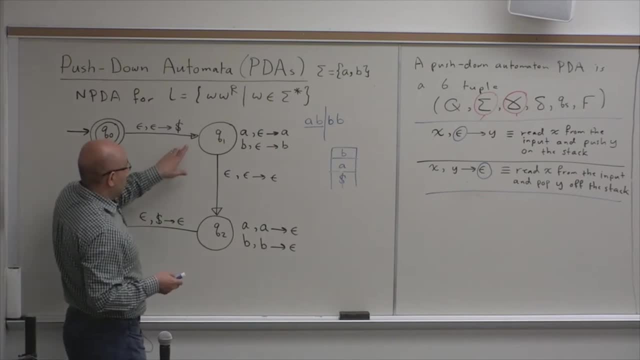 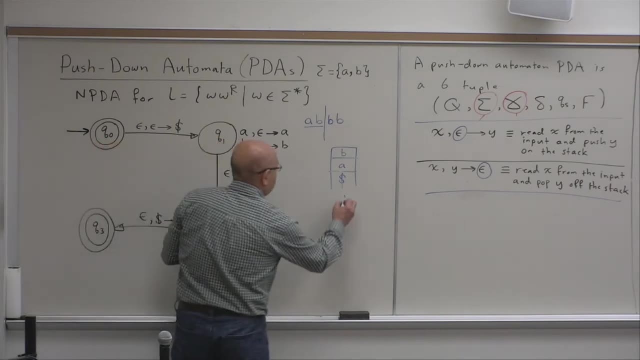 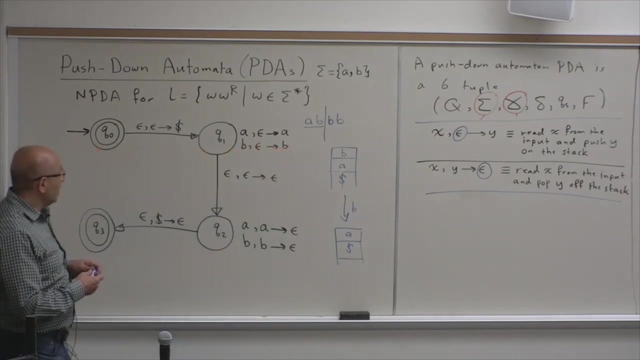 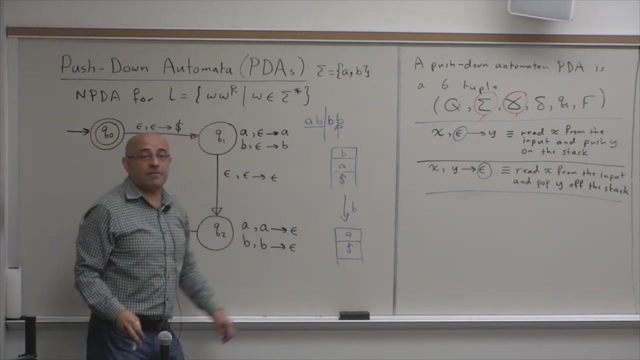 that you can get this accepted. Of course you'll put this, you'll push and you'll get this. Then, when you pop, you pop a B and you will get A dollar sign. Okay, Now you have a B in the input and you have an A at the top of the stack. 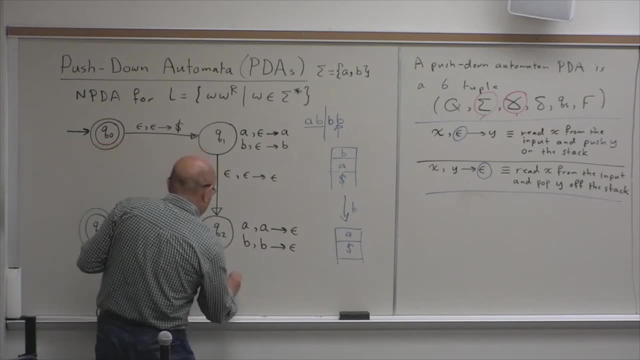 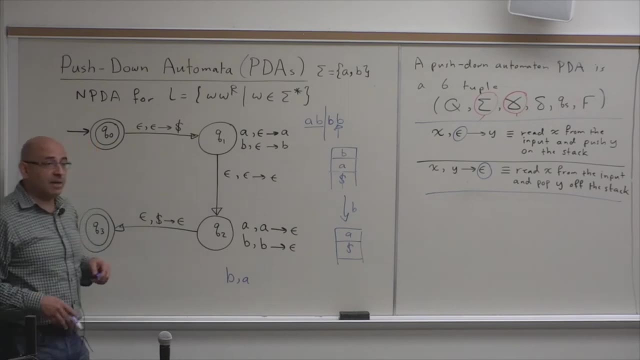 So you need a pair, a matching pair. with what BA? right, But you don't have a BA, So BA is reject, BA go to a trap state. You have an AA and you have a BB, which is a way of expressing the fact. 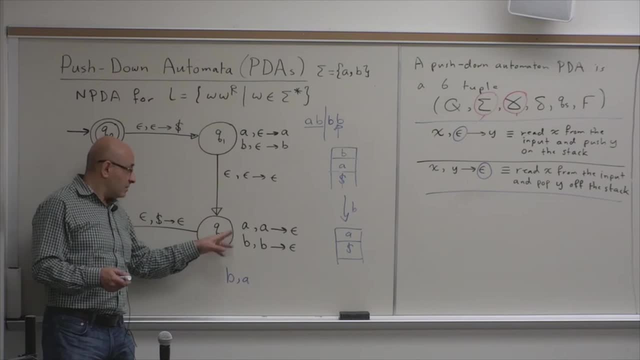 that what I put, What I pop, should match what has been pushed in order for the string to belong to this language, Right? So if I get a BA or an AB- a mismatch- then I reject. Do you see how this is going to accept the strings that belong to the language? 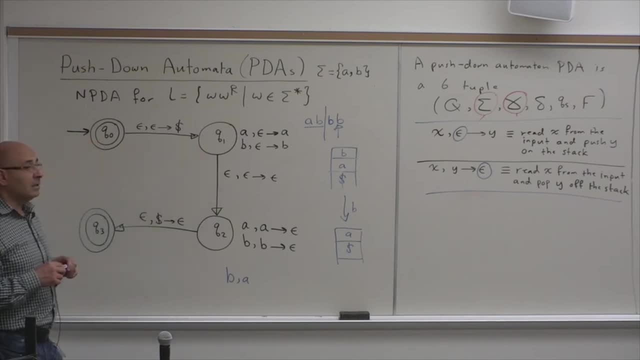 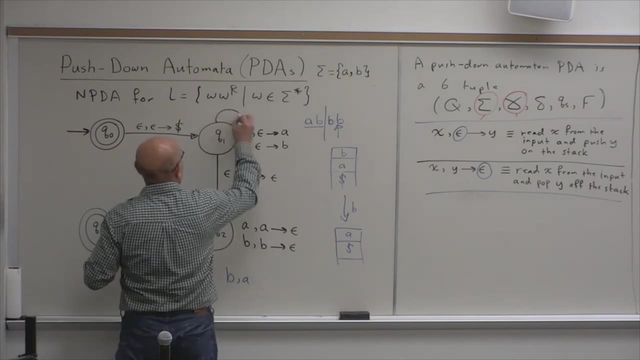 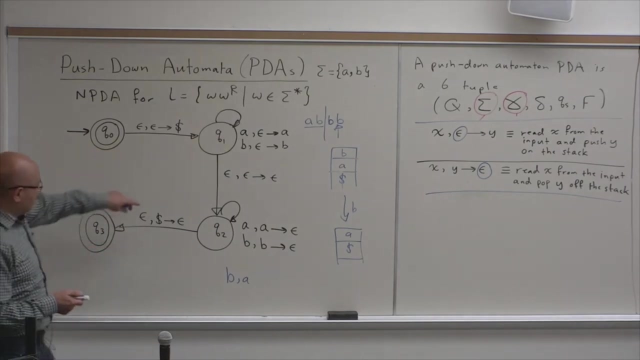 and reject the strings that do not belong to the language. Yeah, Yeah, sure, Yeah, So in fact both Q1 and Q2.. Thank you, Both Q1 and Q2,. you have a loop so you can stay in these states looping. 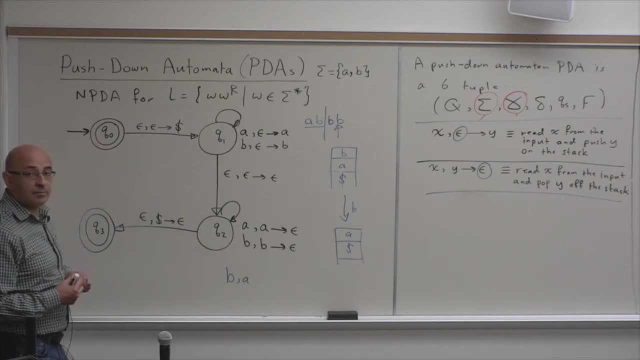 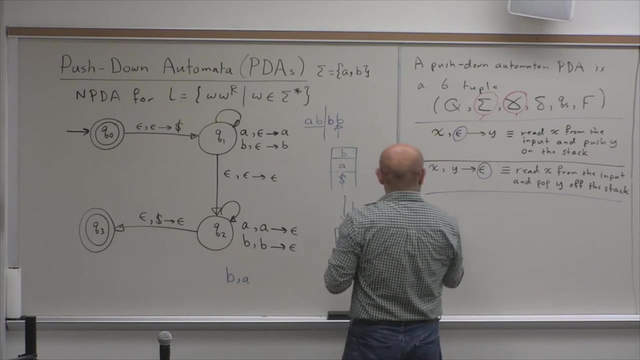 Yeah, thank you. Any questions? Okay, So let's write just to the. you know the formal description of this In this case. for this, our Q is equal to Q0.. Q1,, Q2, and Q3.. 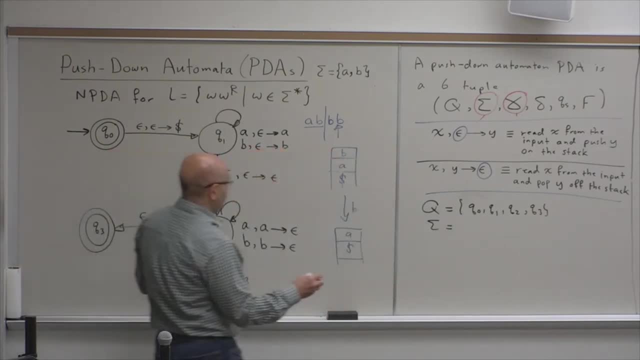 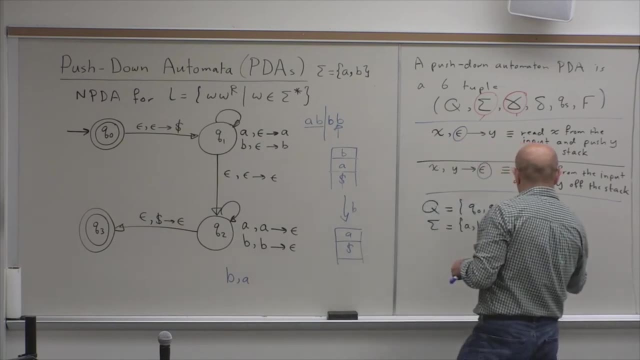 Our sigma is equal to A and B. What's our gamma? Is it really Our gamma? what can we put on the stack? We can put an A or a B Dollar sign Or a dollar sign. So this is a symbol that belongs to the stack. alphabet. 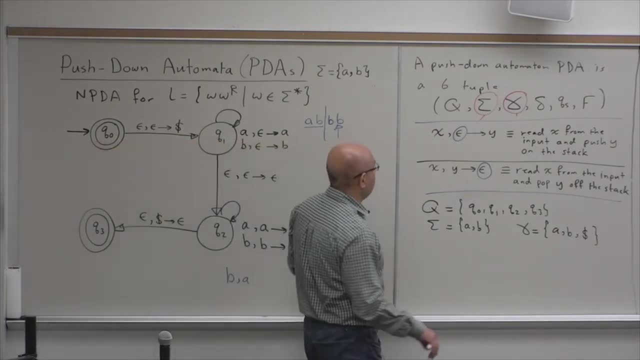 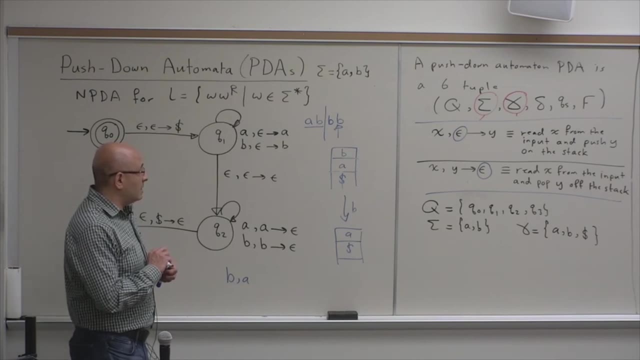 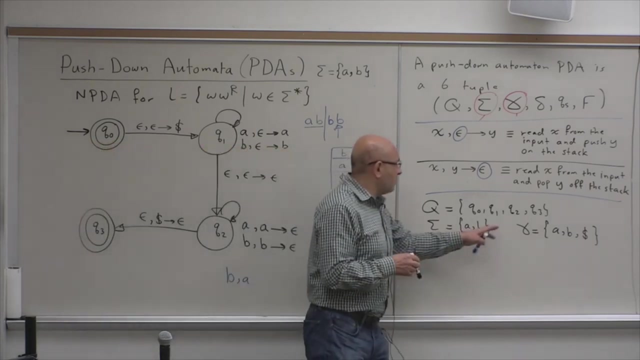 and does not belong to the stack? It belongs to the input alphabet. Will there be cases where it's not a sigma union dollar sign? Sigma union in general? yeah, keep it general. I don't think we'll do examples of that. 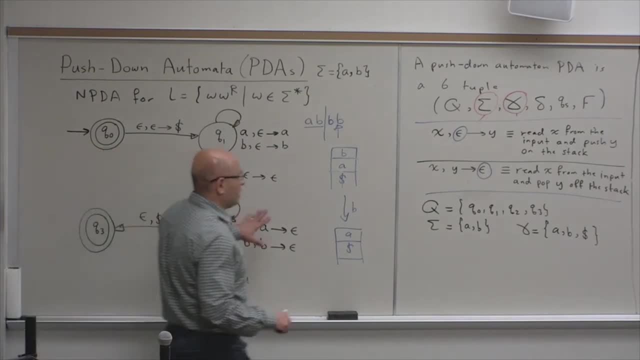 But in general you can put anything, So you can put anything on the stack in general to keep it general. But I don't think we will see examples of that. In fact, we will not see very many examples of PDAs. 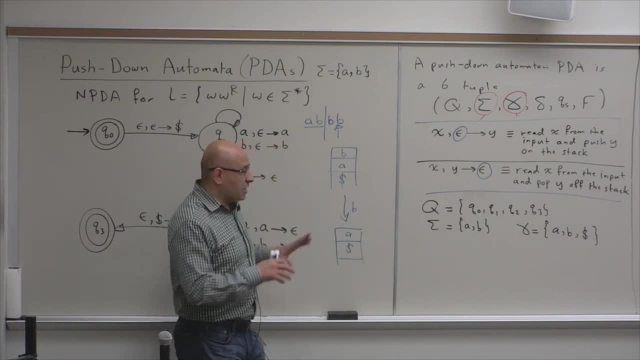 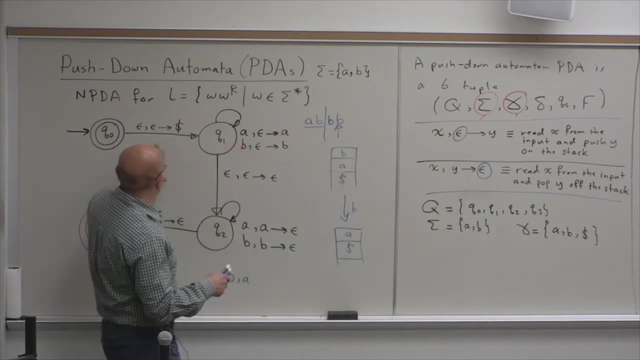 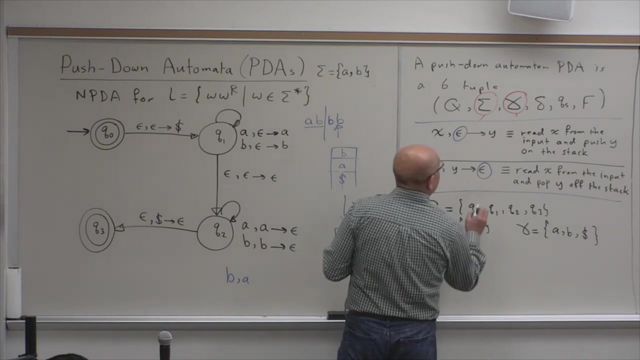 So it's, but in general you can put anything. This alphabet can be totally different than this alphabet in general. And you know, delta is defined by these transitions And QS is equal to Q0.. And F is equal to what?